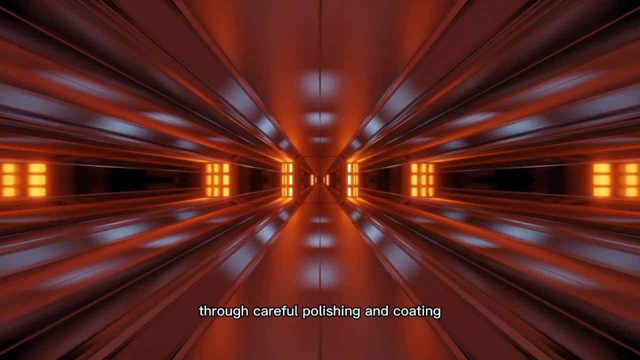 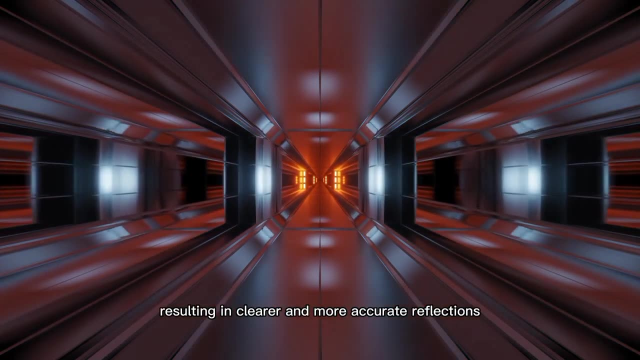 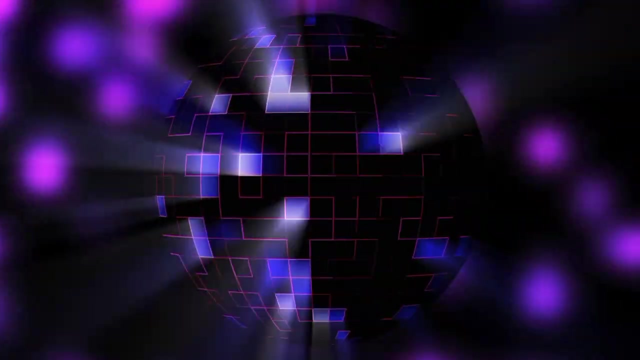 reflection depends on the smoothness of its surface. Through careful polishing and coating, imperfections are minimized, enabling smoother surfaces that reflect light more efficiently, resulting in clearer and more accurate reflections. The choice of reflective material plays a crucial role in mirror performance. 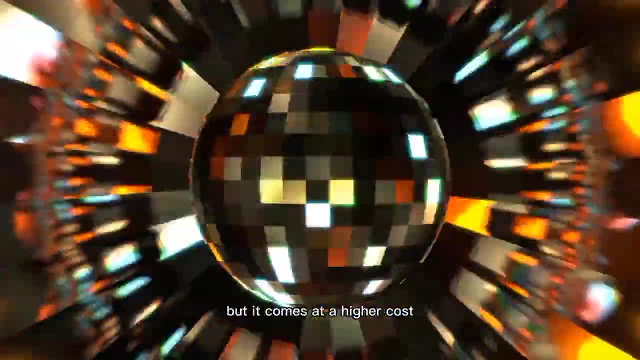 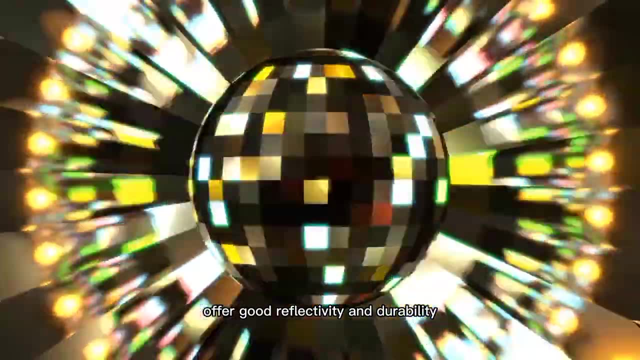 Light is known for its exceptional reflectivity across various wavelengths, but it comes at a higher cost and is prone to tarnishing. Aluminum mirrors, on the other hand, offer good reflectivity and durability at a more affordable price. One intriguing aspect of mirrors is their ability to 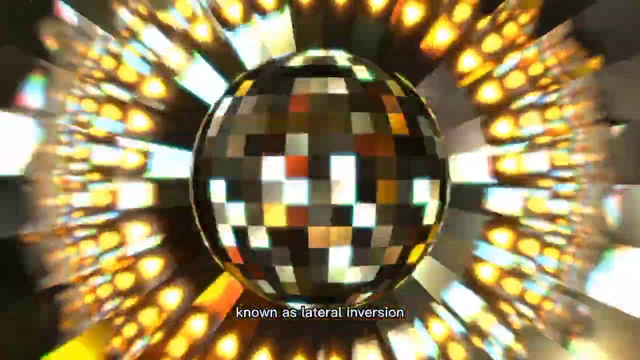 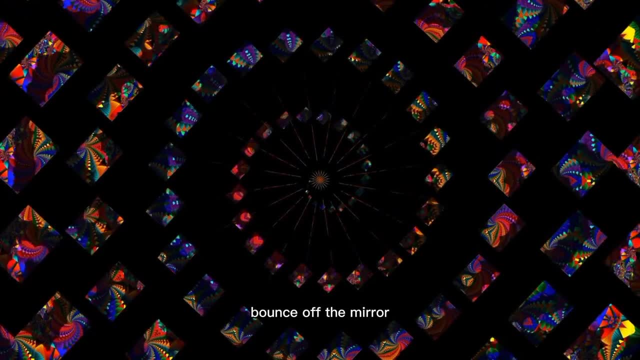 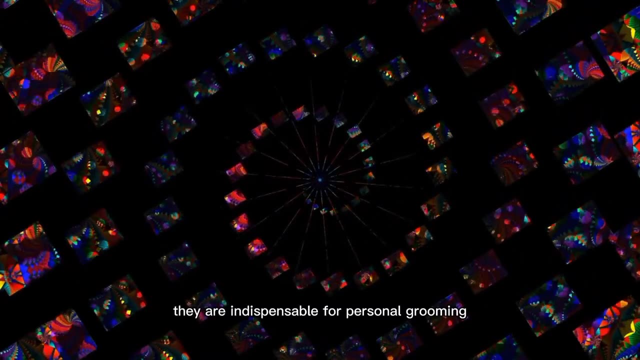 horizontally flip images. This phenomenon, known as lateral inversion, means that the left side appears on the right and vice versa. It is a consequence of the way light rays bounce off the mirror and are reflected back to our eyes. Mirrors find widespread applications in our lives. They are indispensable for personal grooming. 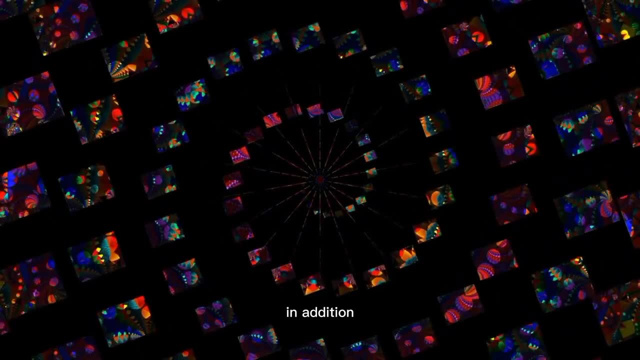 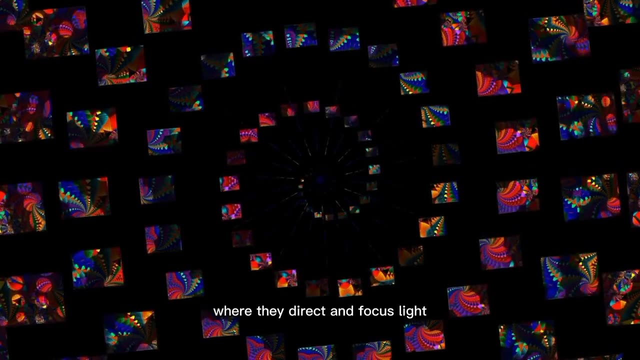 providing accurate reflections of ourselves. In addition, mirrors play crucial roles in optical devices such as telescopes and microscopes, as well as photography, where they direct and focus light. They are also utilized in architecture and interior design to create an illusion of space and. 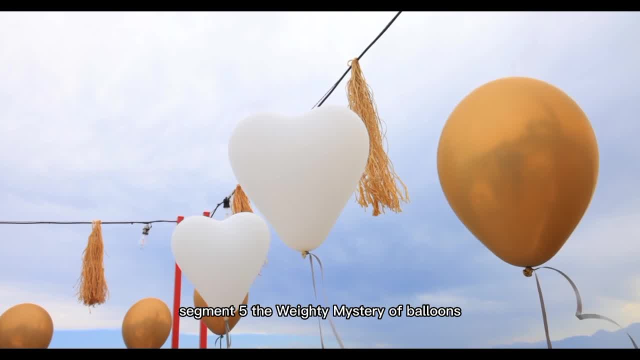 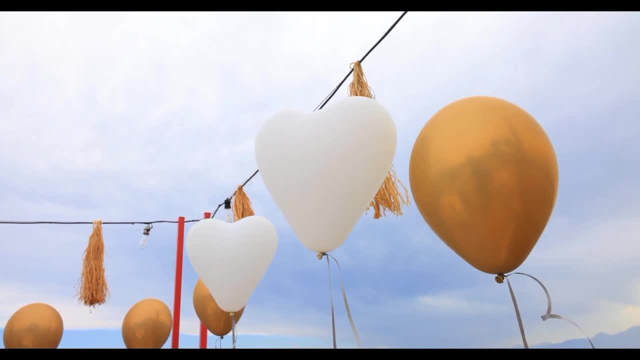 enhance natural light. Segment 5, The Weighty Mystery of Balloons. Floating Balloons have a captivating ability to float in the air. Mirrors are used to create and enhance natural light. The secret lies in the fascinating science of buoyancy, which involves the interplay of gases and densities. 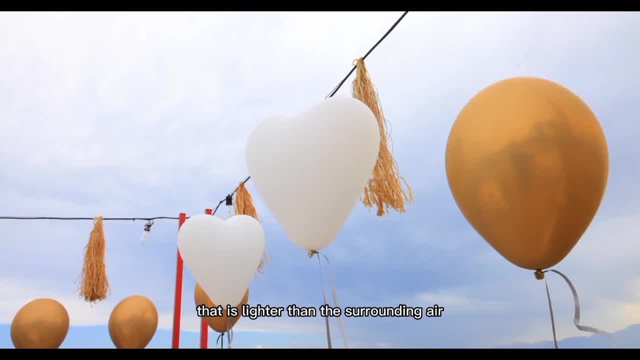 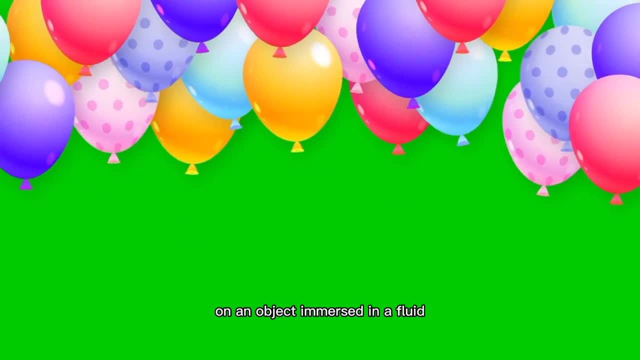 When a balloon is filled with a gas that is lighter than the surrounding air, such as helium, it becomes buoyant. Buoyancy is a result of the upward force exerted on an object immersed in a fluid opposing the downward force of gravity. This force is governed by Archimedes' principle, which states: 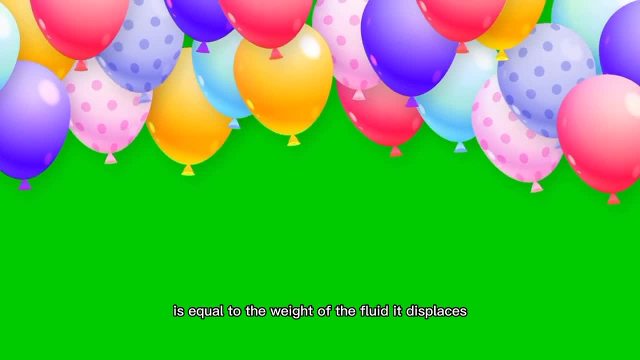 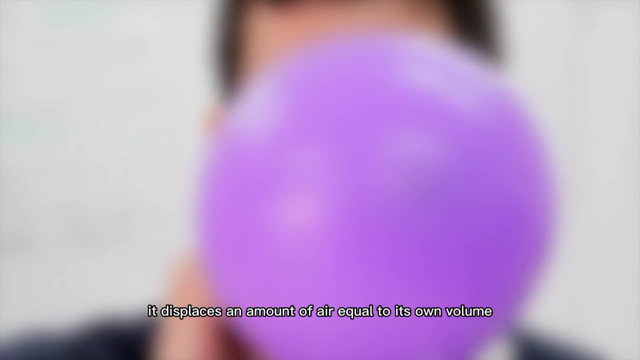 that the buoyant force on an object is equal to the weight of the fluid it displaces. In the case of a balloon, as it fills with lighter-than-air gas, it displaces an amount of air equal to its own volume. This creates an upward buoyant force that exceeds the weight of 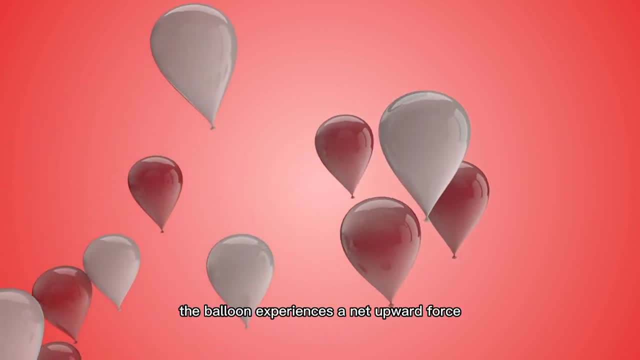 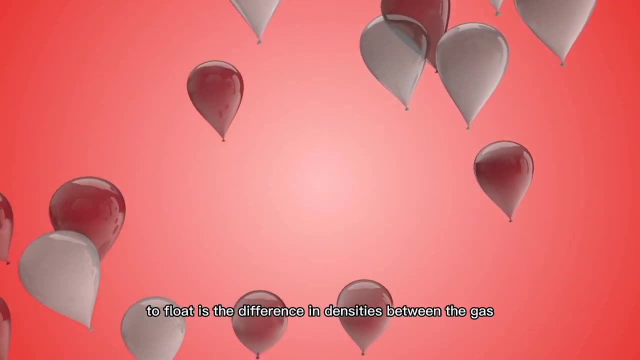 the balloon and the gas it contains. Consequently, the balloon experiences a net upward force, causing it to rise and float in the air. The key factor enabling balloons to float is the difference in densities between the gas inside the balloon and the surrounding air Helium.